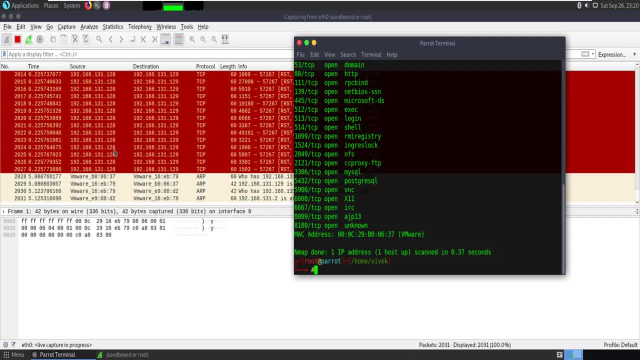 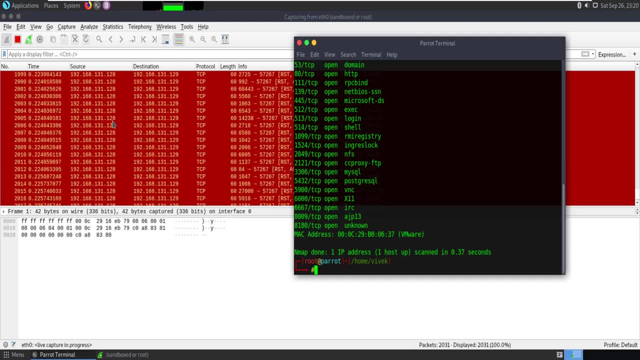 128 is the source IP and 128 belongs to the metasquare table. 129 belongs to my parrot. Okay, so this is my IP: 192.168.131.129.. okay, so you can see one source and destination. all all these things now. 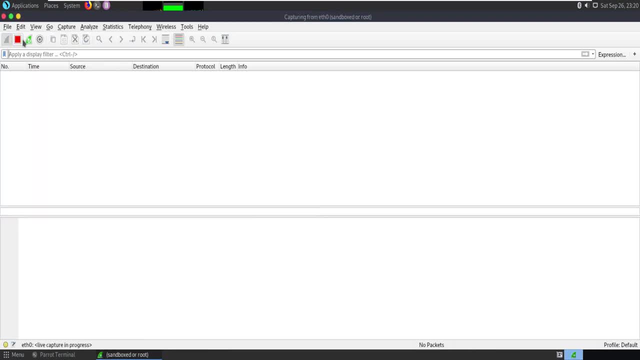 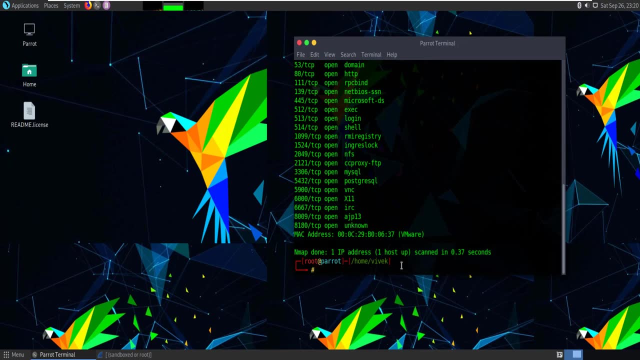 what I'm going to do in this practical. I am going to capture, spoof IP. okay, so I will spoof my IP. so, IP spoofing, there is one simple technique, what I can do: nmap-e. then you need to choose your adapter. okay, so Ethernet adapter I am. 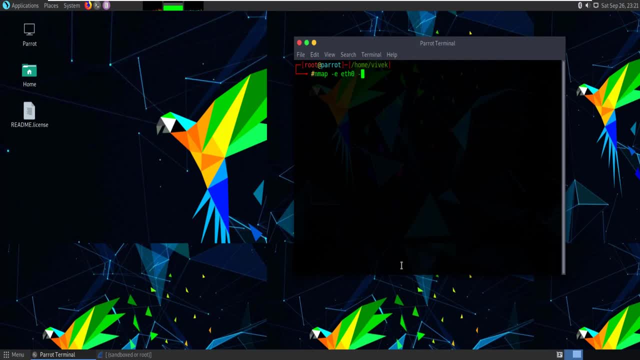 choosing, then I- capital S, then what IP you want to choose. for example, I want to choose this IP 131 or 113.15.102.1,15. okay, so I'm just using any random IP. then you can choose the destination. destination is my. 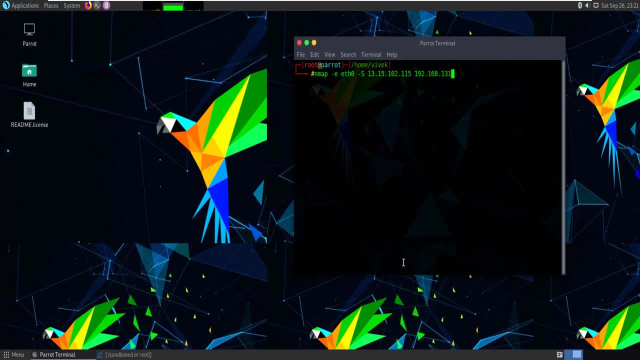 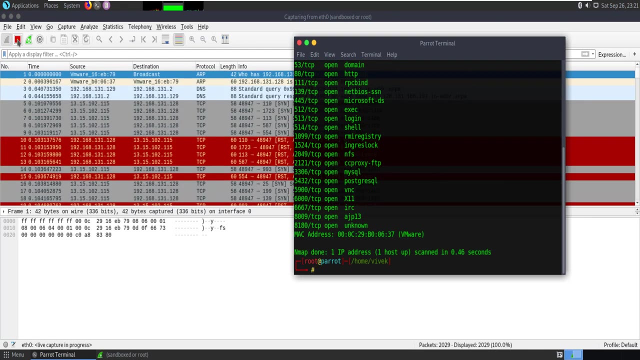 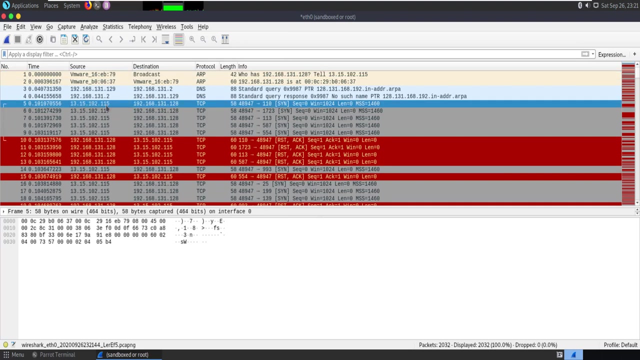 metasper table. so 192.168.131.128, it okay. 192.168.131.128, dot 131, dot 128, okay, so let me start capturing. so it is started. enter, okay, so results even you can see. so what is the source ip? here you can see 13.15.102.115, right, so this is the source ip and 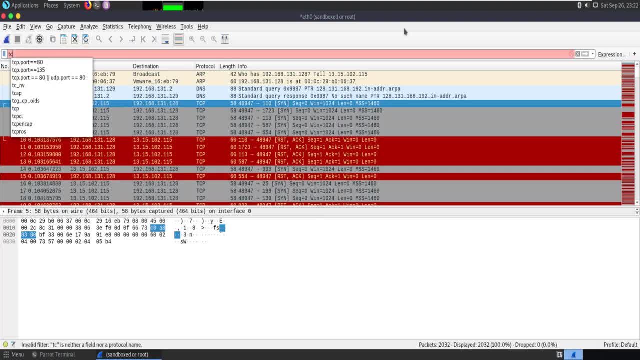 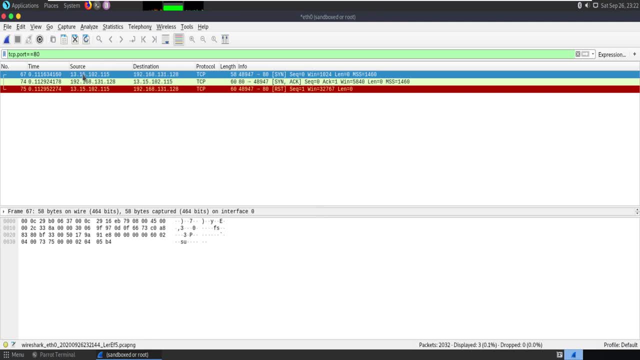 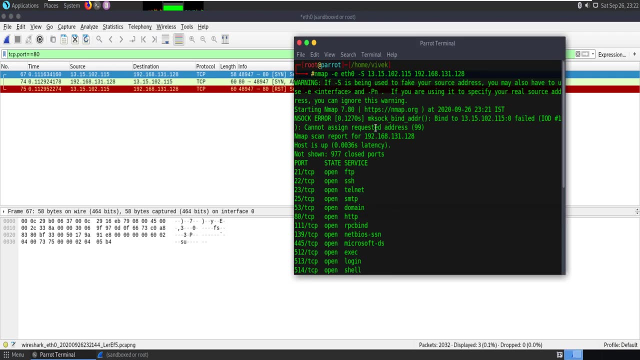 this is the destination ip. so if i'm filtering the port, so tcpport equals to equals to we. you know that 80 port number is open. so what is the source ip? uh, request generated from this fake ip. okay, 13.15.102.115, that fake ip we have created. even you can see 13, 13.15.102.115. so this is the spoofed. 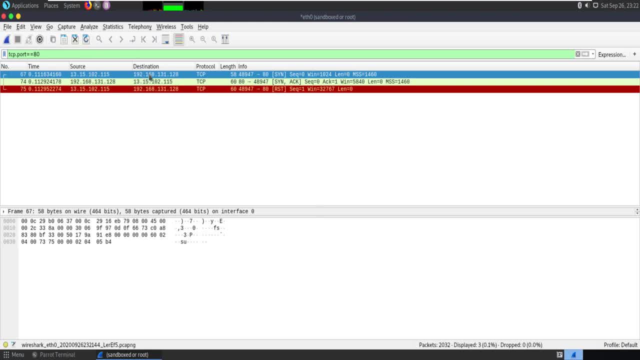 ip. so from this spoofed ip this request is going to the destination. then destination is replying to this spoofed ip. only you can see this is the metaspheritable ip 128. so metaspheritable is replying to this is spoofed ip. okay, cincinnati rst. so this spoofed ip is then acknowledging to the destination. so 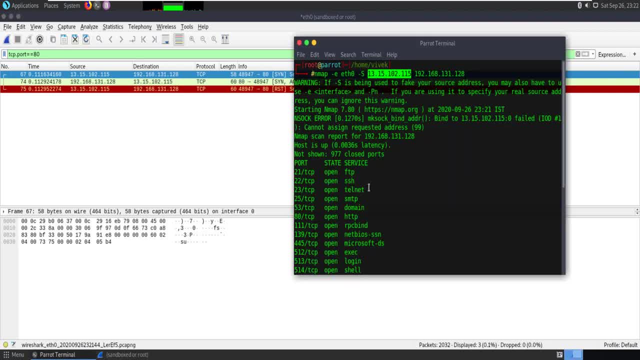 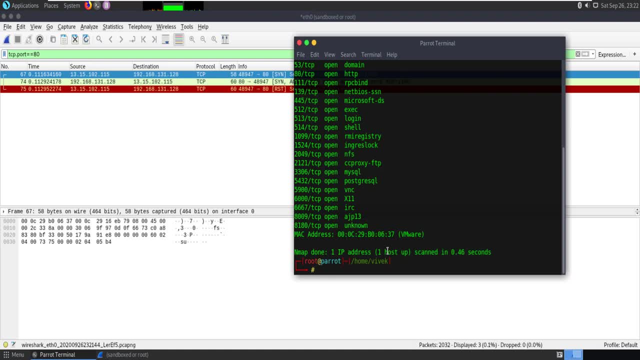 this is how scanning is being done. okay, so this is the one technique how you can spoof your ip. i hope it is very clear to you. so second technique: now we are going to check second technique and second technique. second technique is even more interesting in the second technique. 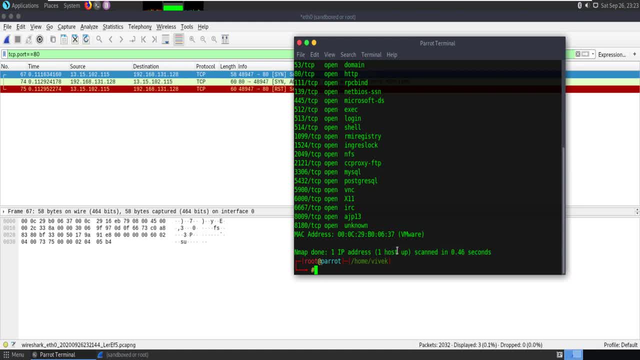 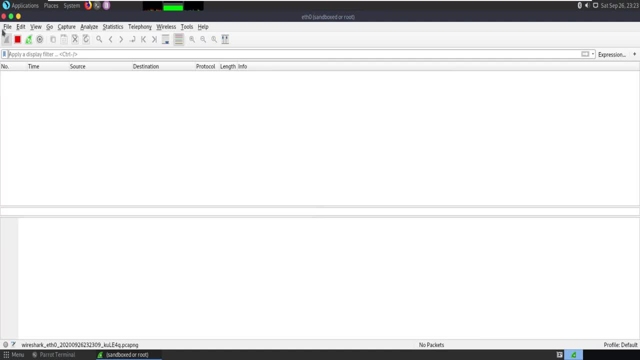 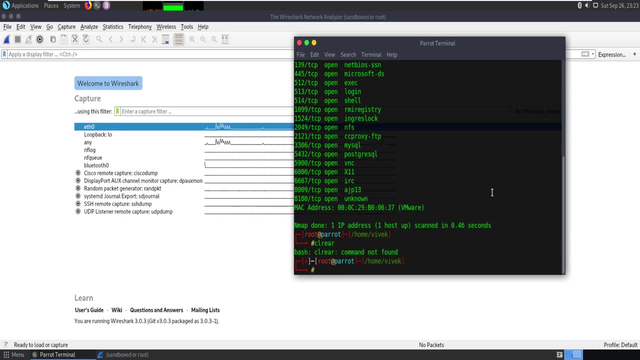 what we are going to do now. here you have used only one single fake ip. now what i'm going to show you? i'm going to show you multiple fake ids, ips at once. okay, so how you can do that. so let's do that clear and sorry. okay, so command is end map. okay, then uhrock. 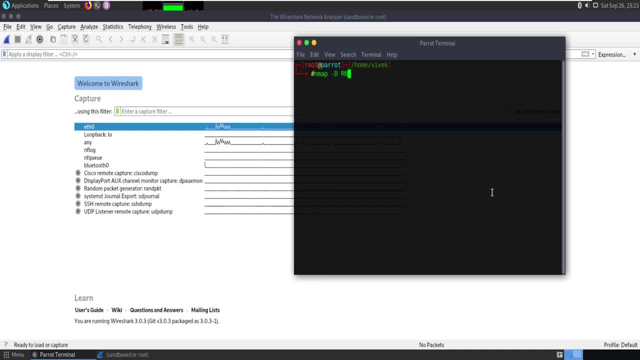 capital d. capital d will be used for the decay of the ip address. then random: how many random ip address you want, and you want How many random IP address you want to choose. Then that is a column and 10.. Okay, so I want 10 random IPs generated from as a decoy IP. Okay, then you can choose your target. So my target is 192.168.131.128.. This is IP of the MetaSquare table. 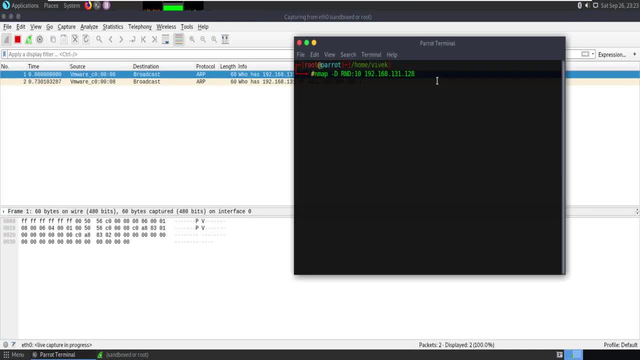 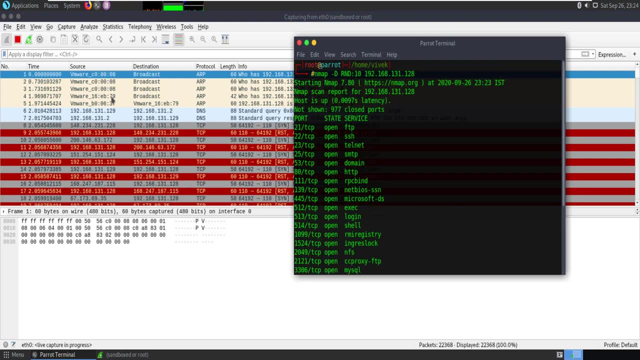 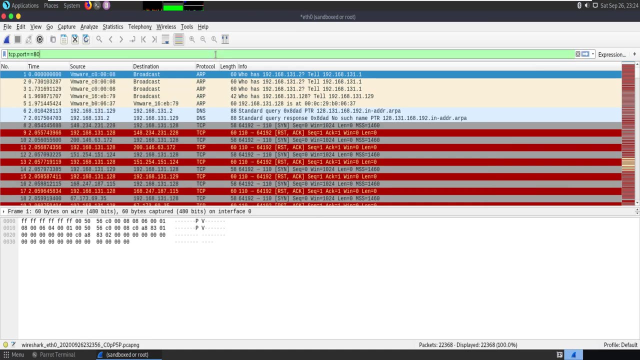 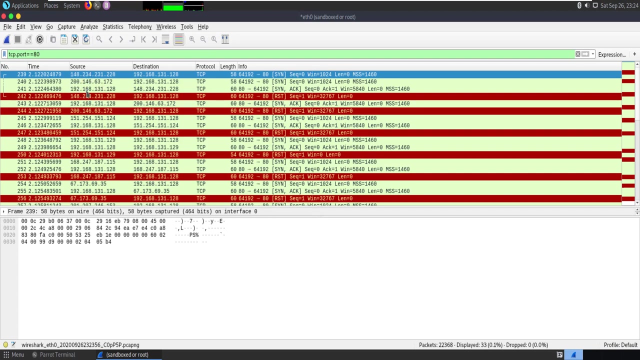 Okay, so let me start capturing and hit enter. So, as you will see, okay, result is in front of you. So these are number of ports. So now let me show you again. filter tcpport equals to equals to 80. So here you can see. can you see source IP 148.200.192.192. is the response actually SINAC? Okay, so SIN. So only SIN packet. I want to. 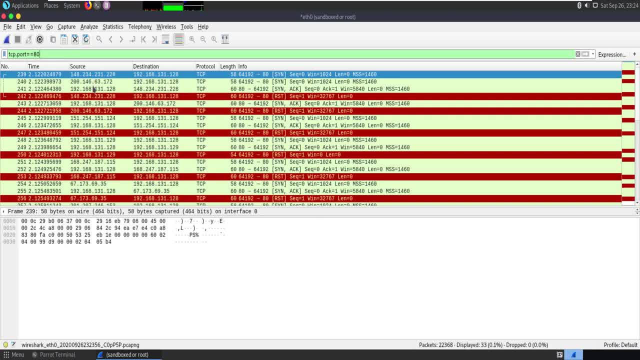 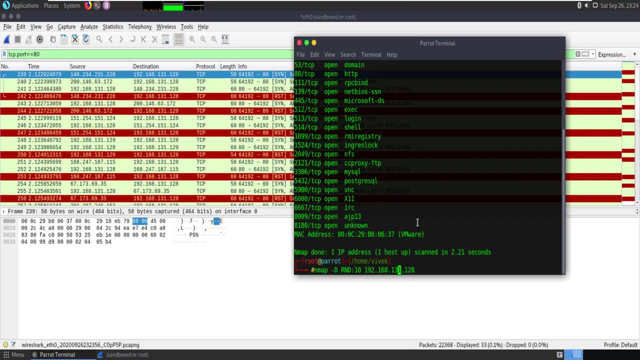 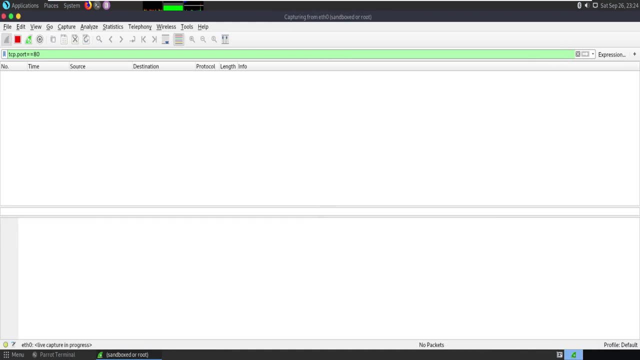 Check. Okay, so you can see 1,, 2, 3.. If you will count, so there are 10 random IPs are there? Okay, so it means 10 random IPs we have generated. If you will increase that count. Okay, so, for example, if you will increase that count to the 100.. So here you can make it 100.. Restart the capturing, Then hit enter. 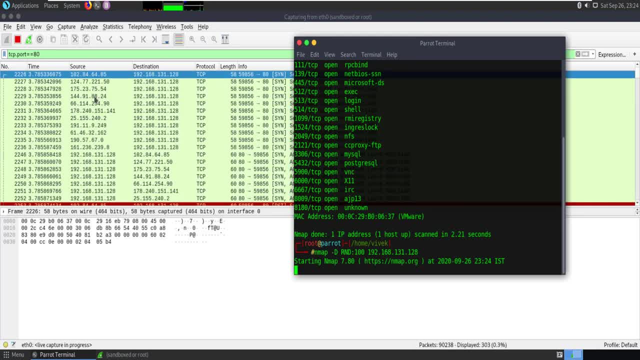 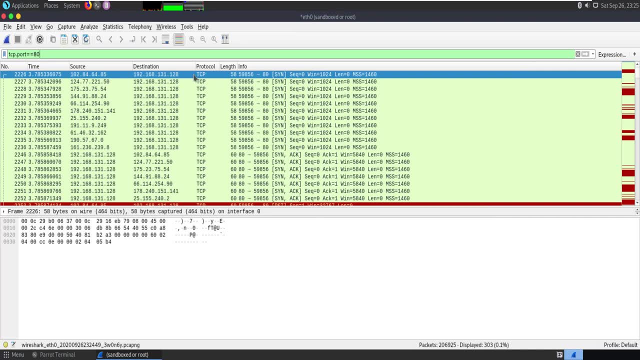 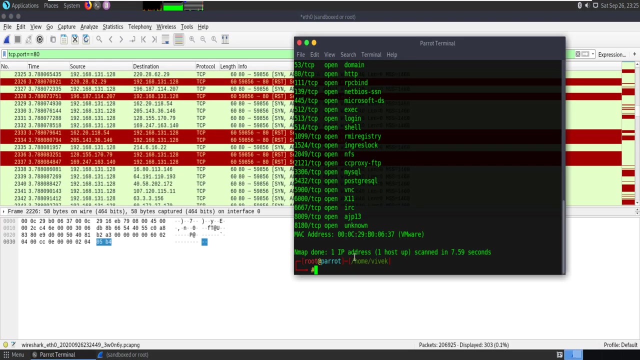 Okay, so you will see 100. 100 random IPs will be generated this time. Okay, hundreds of random IPs. So it would be very difficult to trace. even You can see 102.84.64.85.124.175.144 random IPs. Okay, so 100 random IPs are generated now, this time. So even you can check. Okay, so this is the decoy of this IP. So here in this lecture we have discussed IP spoofing and the decoying of the IPs. 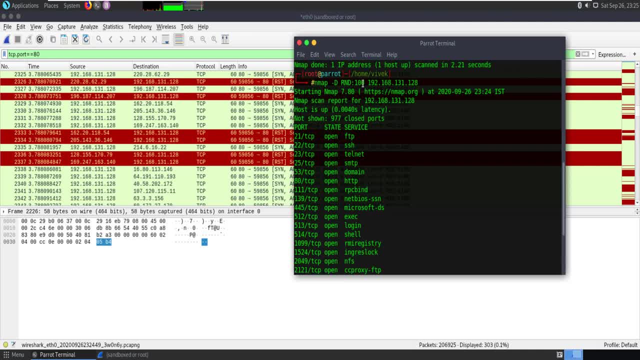 Okay, so with this IP decoy, you can choose any number of random IP addresses, So I hope you have enjoyed this session. Please like, subscribe and share my channel. Thank you, Thank you everyone.